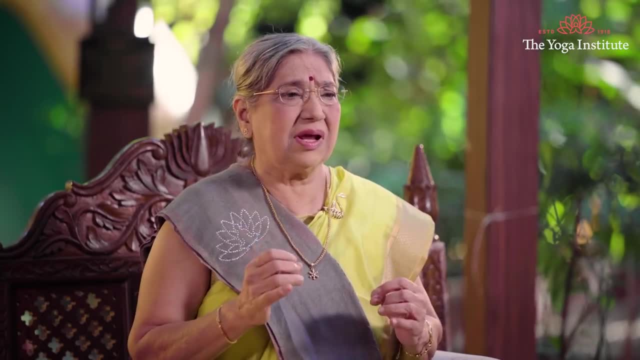 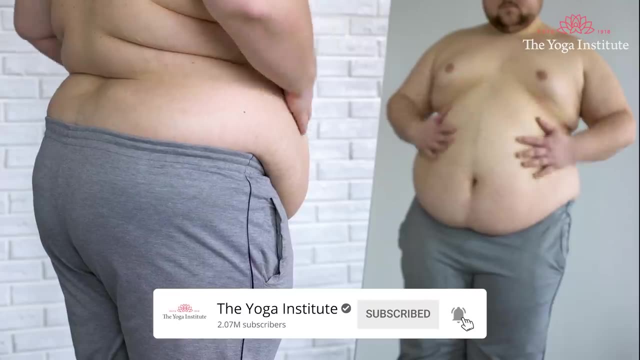 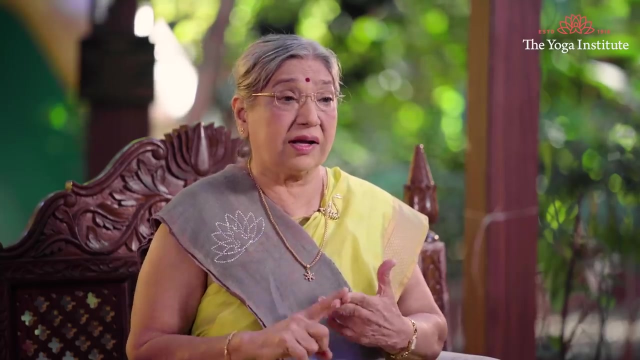 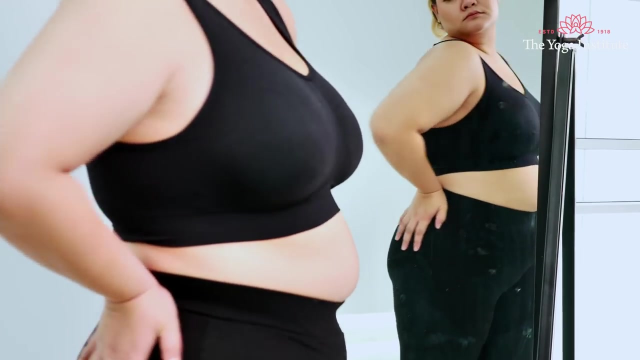 Namaskar, Learning to accept and embrace the structure, the shape of your body is first thing you should do. This will stop negative thoughts about your body from upsetting you. Your goal should always be to attain healthy and toned body through the right techniques and through the right lifestyle. Women usually face the problems of broader hips. 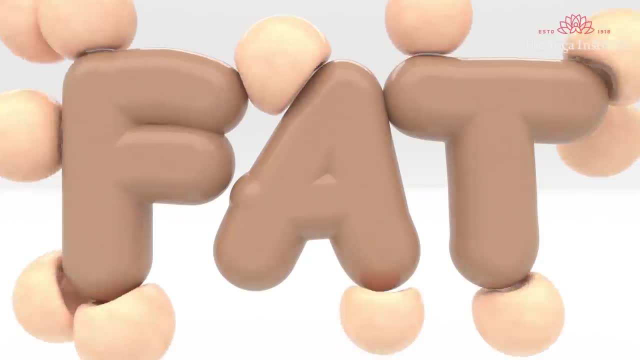 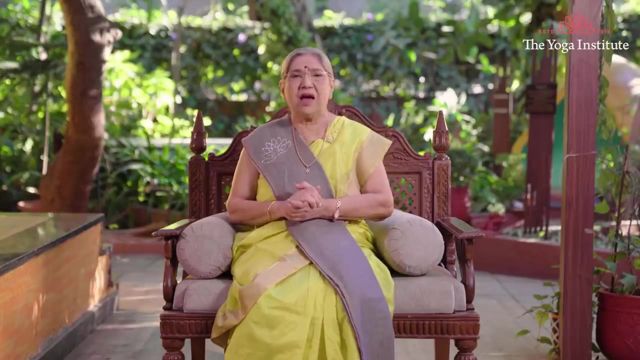 This could be due to the hormone, estrogen, which has an influence on where the fat is stored. especially during pregnancy, Women stores fat around hips, pelvis and thighs, as this acts as a storage of energy which is required for lactation. Today I'm going to share top five. 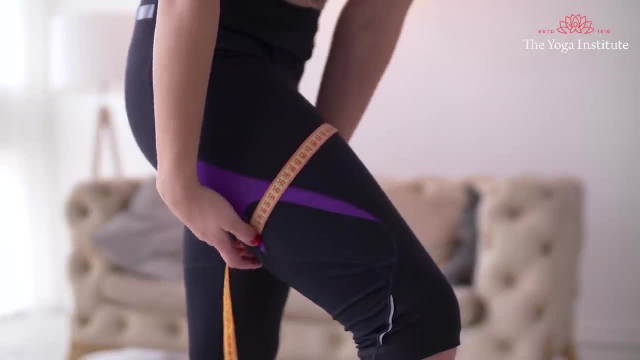 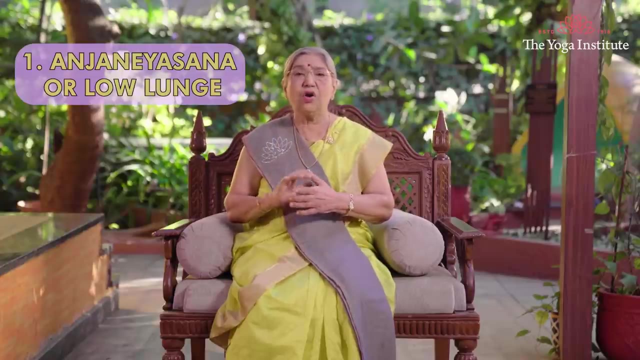 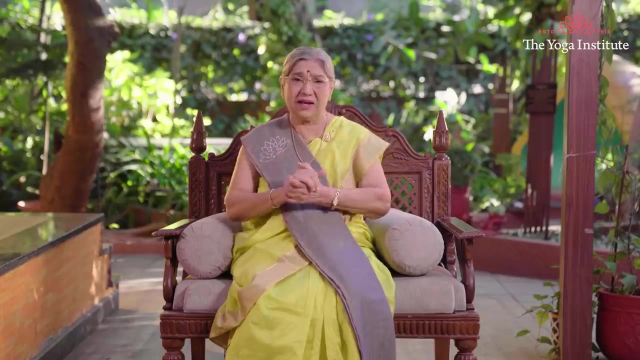 asanas that would help you to lose weight around your waist and will tone your broader hips. First, Anjaneya asana, or low lunge. Anjaneya asana targets more than one muscle group and helps to shed accumulated fat in the lower body region. It engages the hips. 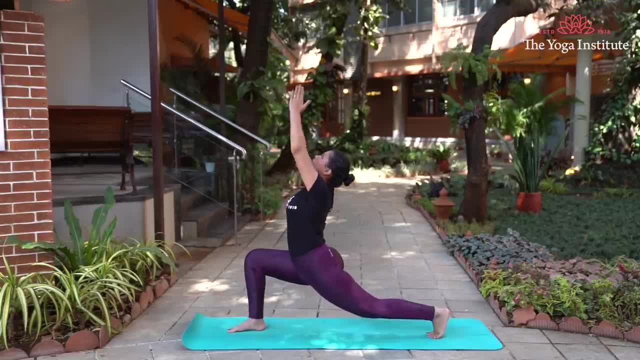 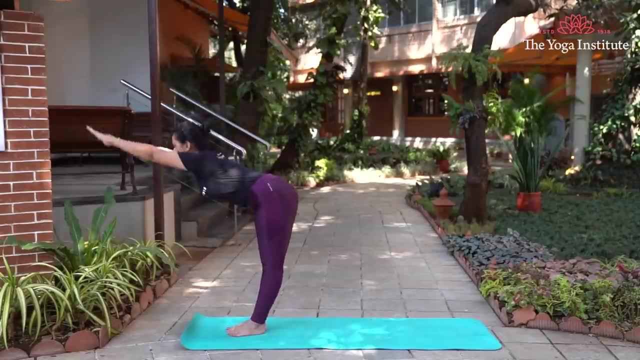 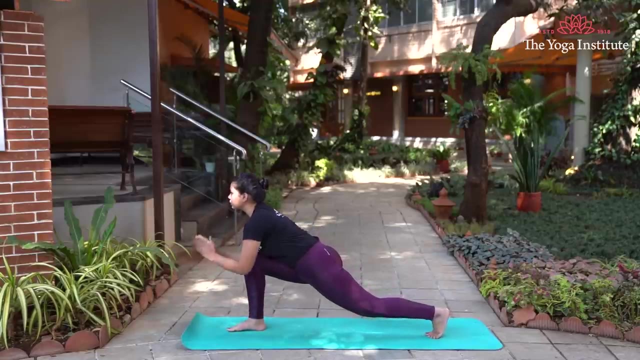 pelvis and the lower body muscles and works and tones the area effectively. Now understand how to do it. Stand straight Now. lower your body down by slowly extending your right leg backward. Try to extend it as far as possible. Your right toe should touch the floor. Your left leg will. 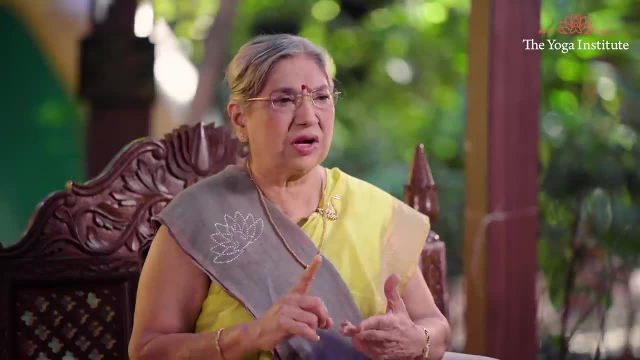 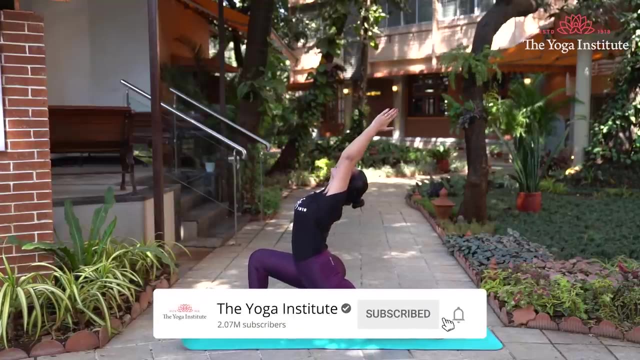 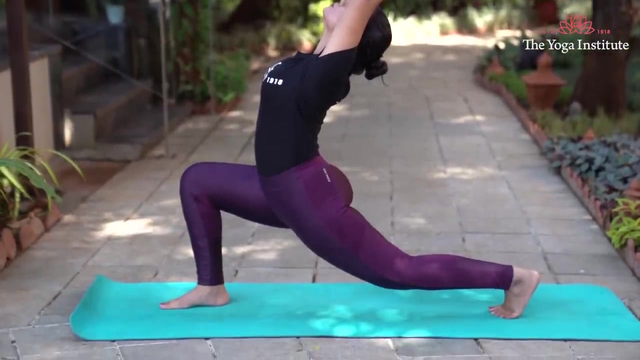 gradually bend from the knee. Make sure that your knee and ankle are in one line Now arch the spine, look upwards and balance the body. Sustain this posture for three seconds and repeat it three, four times. Repeat it on the other side. Second frog pose. 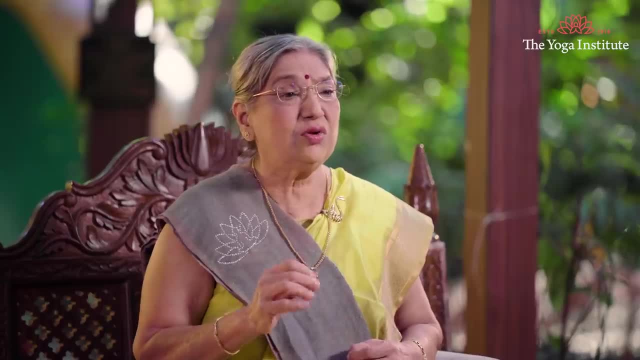 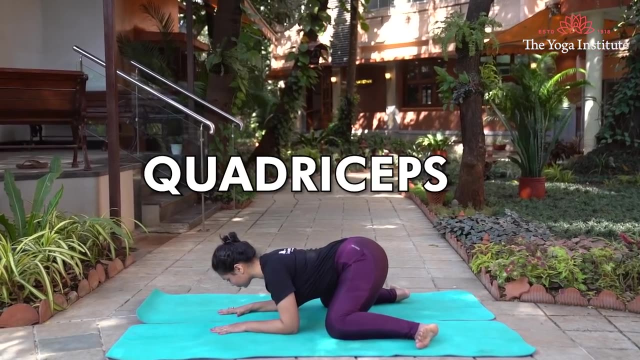 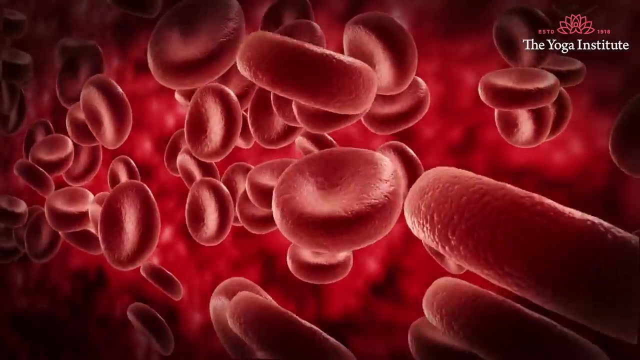 Frog pose is an intense stretch to reduce broad hips. It stretches, strengthens tones and releases tension in your quadriceps, hip joints, hamstrings and glutes. It enhances the circulation of blood in the lower part of your body. Now let's understand how to do this. 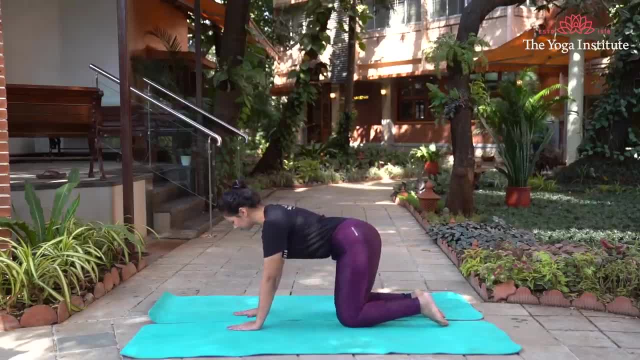 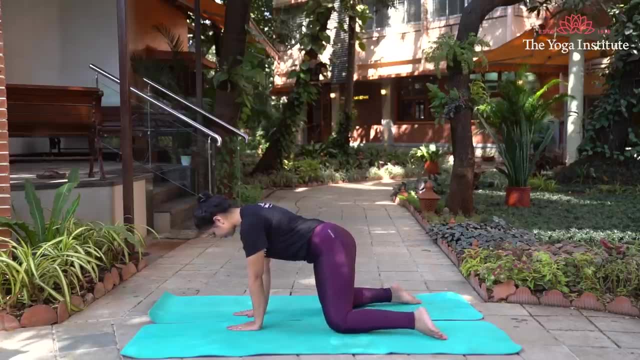 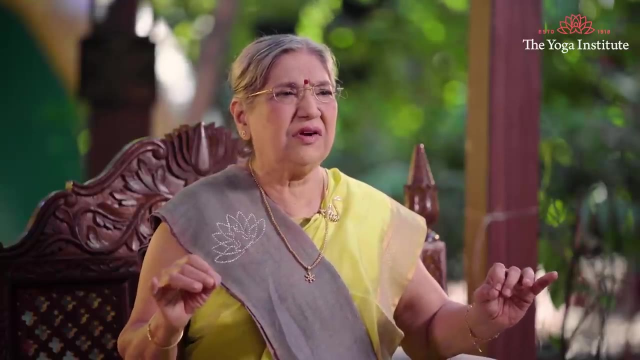 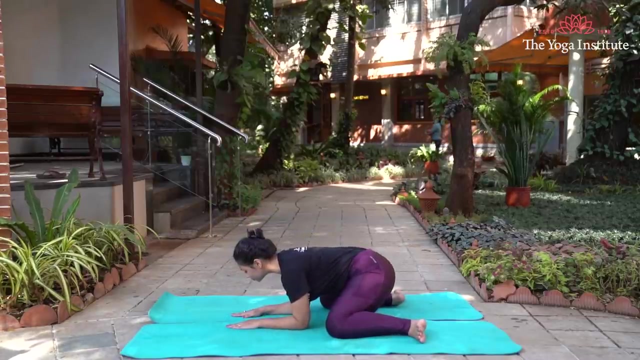 frog pose: Come in a tabletop position on your hands and knees. Inhale and slowly spread your knees outwards. Continue as long as you feel the stretch is comfortable. Stop extending the legs if it hurts you. Now slowly lower down to your forearms with the palms flat on the floor. 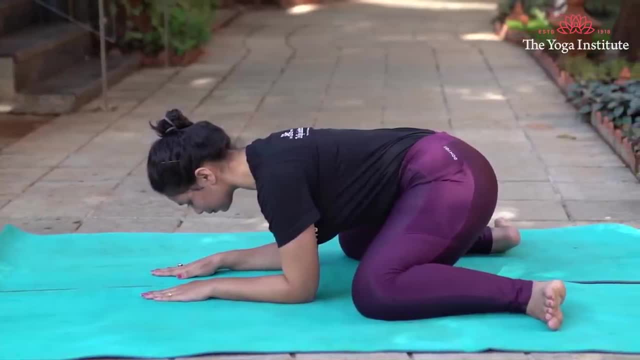 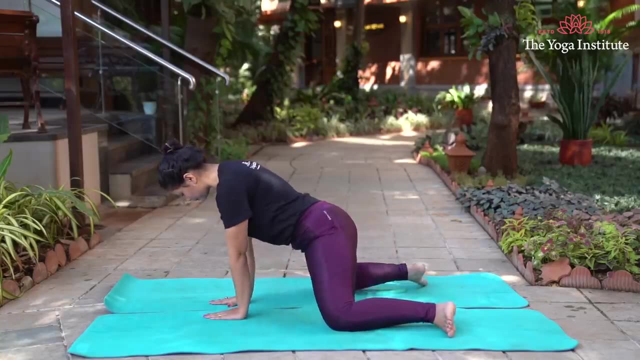 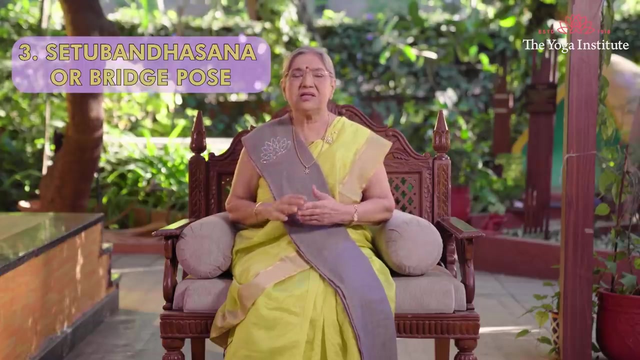 Stay here and breathe deeply for the count of five seconds To release the frog pose. slowly slide your knees together and closer and return to the table In the tabletop position. you can repeat this five times. Third setu bandhasana or bridge pose. 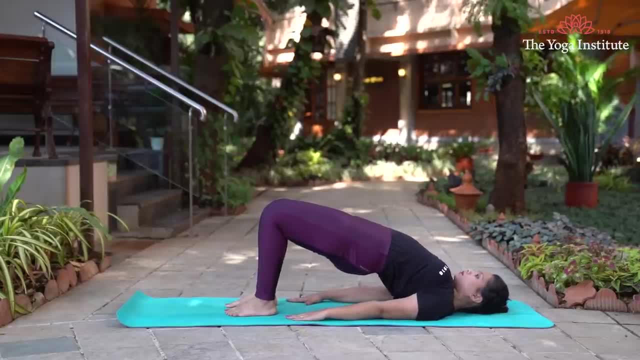 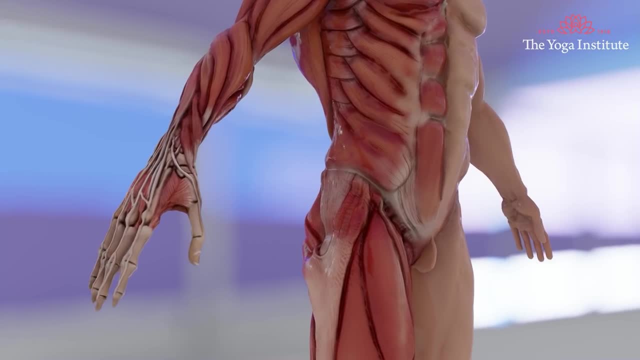 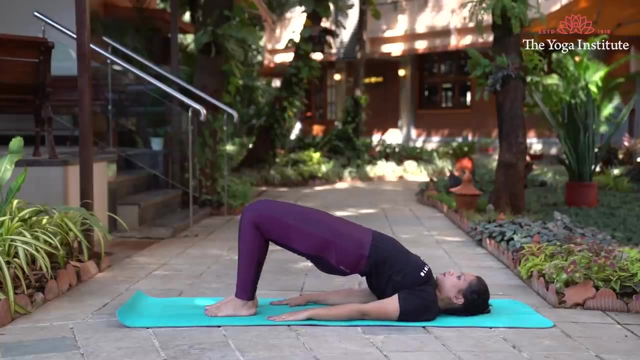 Setu bandhasana is another simple yet super effective asana. It helps burning fat from the hips and thighs. It tones the lower body muscles and strengthens core as well as back. The upward movement gives intense pressure on the hip area. that stimulates the muscles and helps to 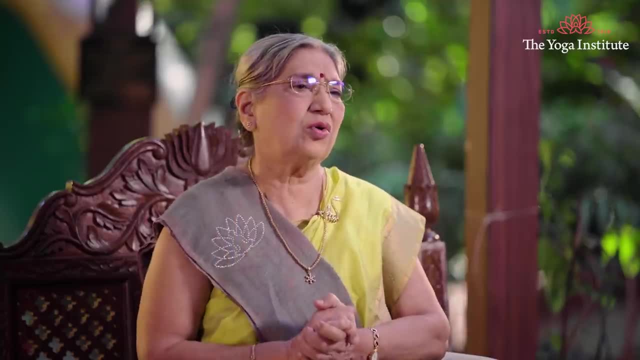 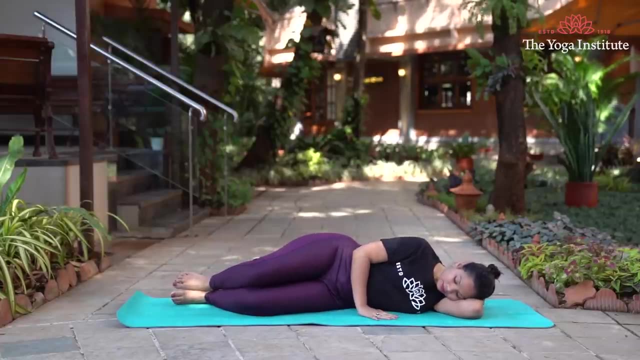 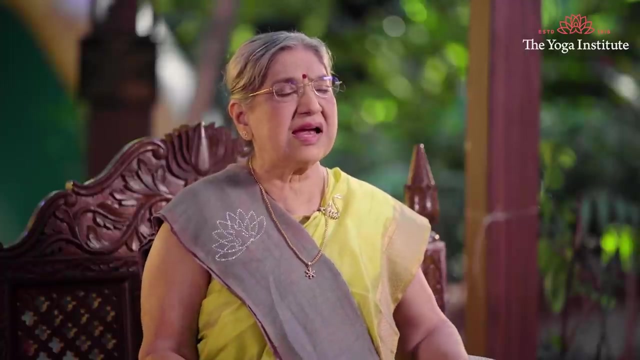 burn the excess fat. Now understand how to do it. Lie down on your back. Pull your feet towards hips. Keep your feet parallel to each other and the knees pointing to the ceiling closer to each other. Place your arms beside the body, palm facing downwards. Now inhaling slowly. lift your 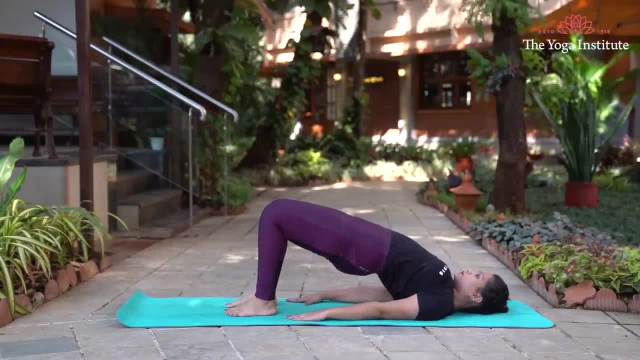 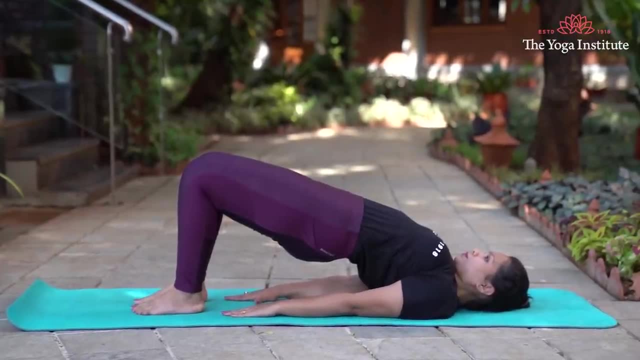 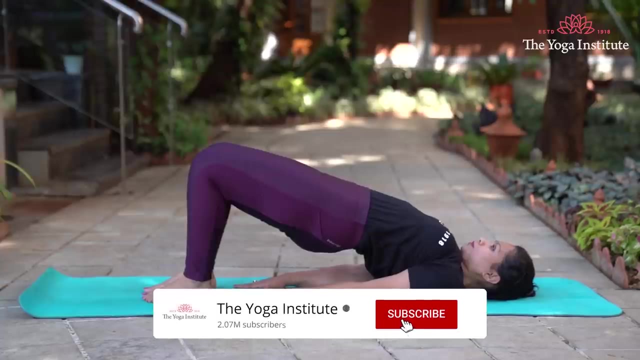 lower back, middle back and upper back off the floor. Your chin will touch the floor Chest. Remain lifted like this. Keep breathing normally and slowly. Hold the posture for 10 to 30 seconds. At that place you can breathe normally and then, exhaling, bring your back. 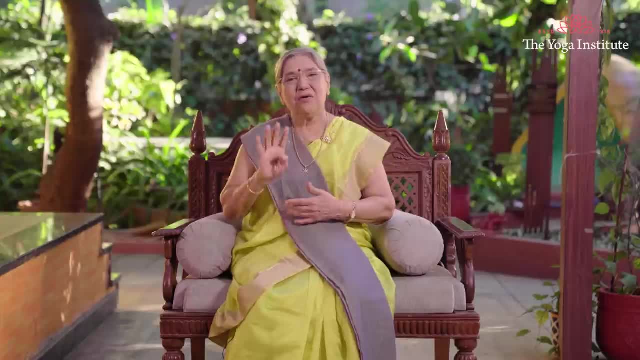 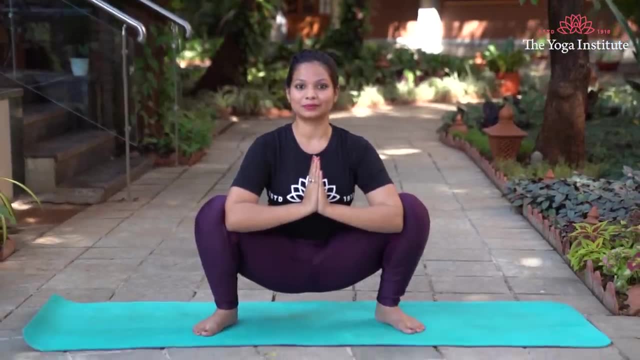 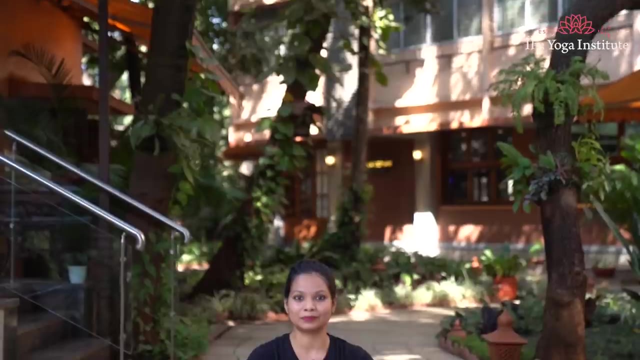 back to normal. You can repeat this five times. Fourth malasana, or garland pose. Malasana is an excellent asana to increase circulation in pelvic region and hip region. This simple asana targets the inner thigh and hip muscles and that really helps. 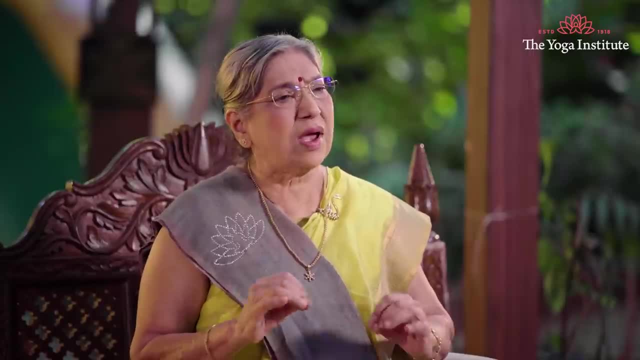 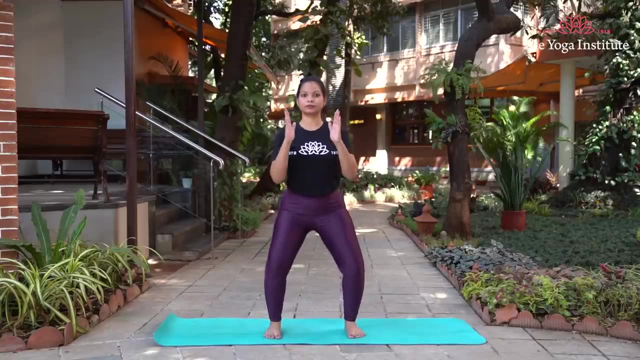 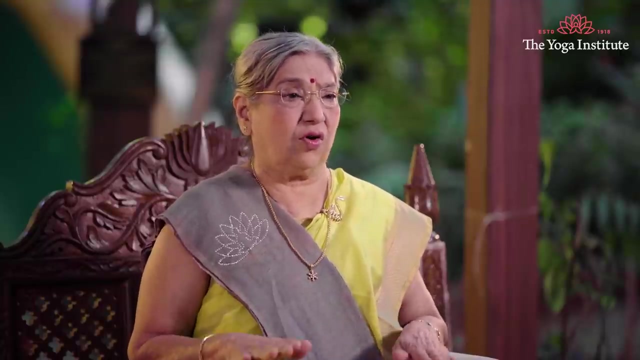 to reduce fat effectively. It also helps to enhance lower body flexibility. Now understand how to do it. Begin with the low squat form with the feet at one and a half feet distance. Try to keep feet flat on the floor. Now spread the thighs as wide as possible. Place both palms. 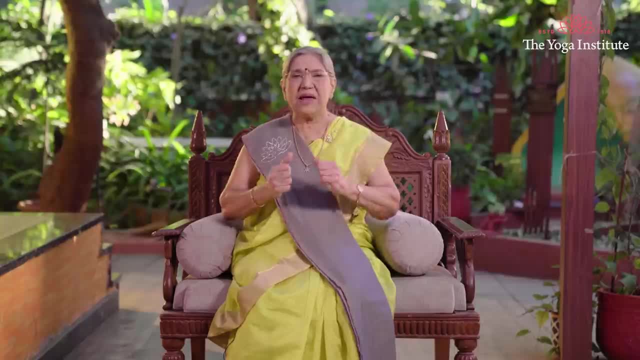 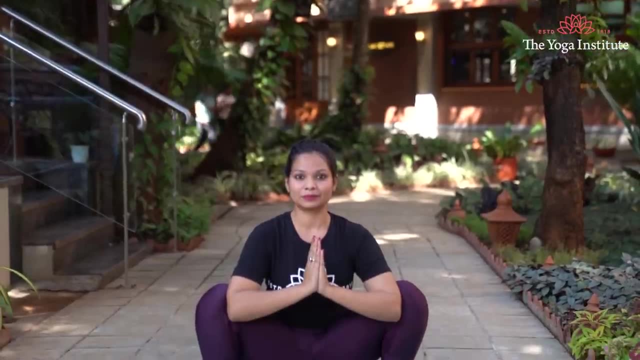 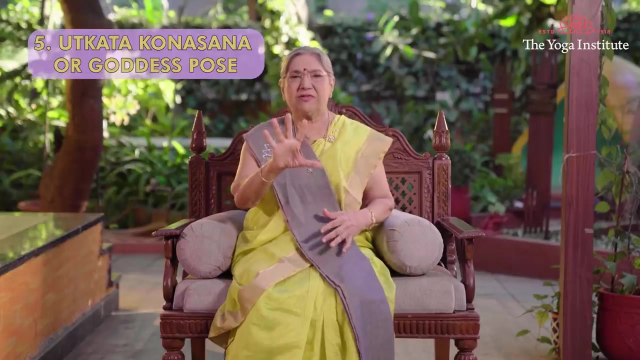 together in front of your chest in namaste position. Press the elbows against inner knees and lengthen your torso at the front. Hold on to this position at least for 30 seconds. Slowly release your position. Do this five times. Fifth, utkat konasana or goddess pose. 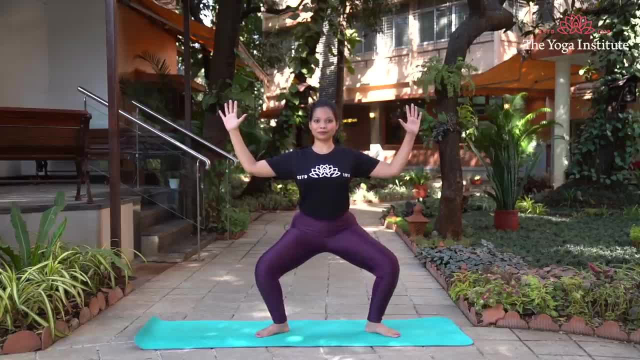 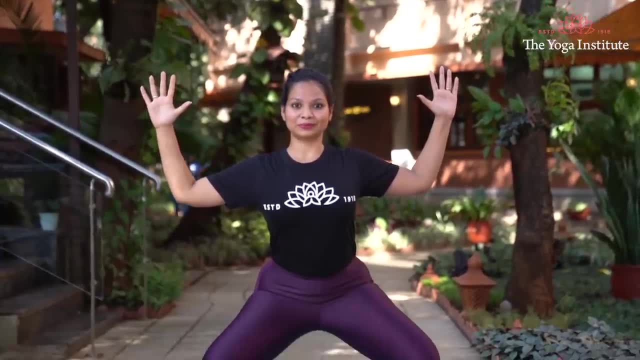 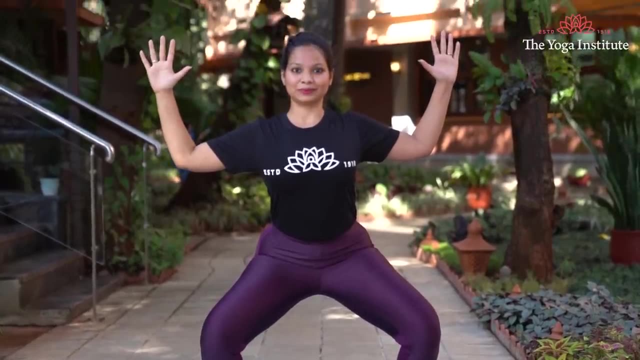 Utkat konasana is an excellent asana to put pressure on hip muscles, Although this asana looks simple, but it can become quite challenging to hold this pose for 30 seconds. When you hold this pose, the quadriceps, hamstrings, hip joint and glutes all get engaged, which helps to tone the 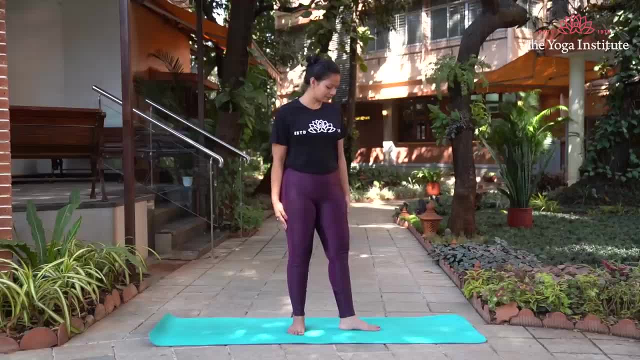 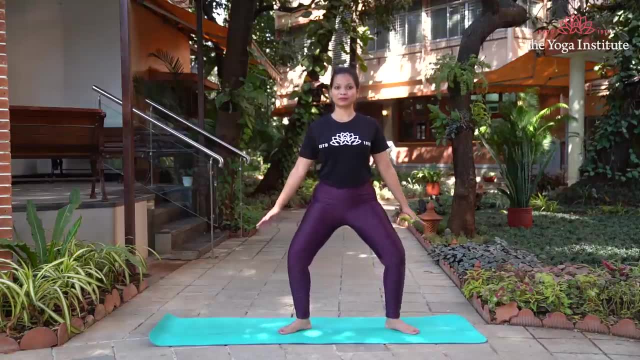 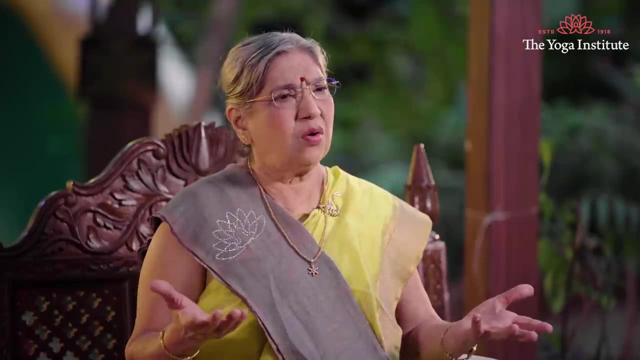 broader hips. Now let's understand how to do it. Stand straight and keep your feet around three feet apart. Now breathe in and bring the hips down while bending your knees and legs. Come down as if you are on the floor, If you are sitting on a chair, or go down as low as you can without losing your balance, Make sure. 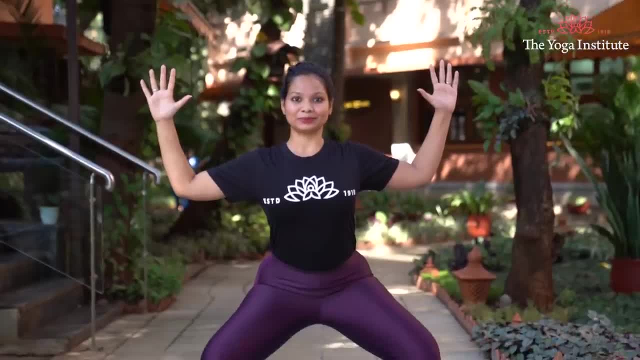 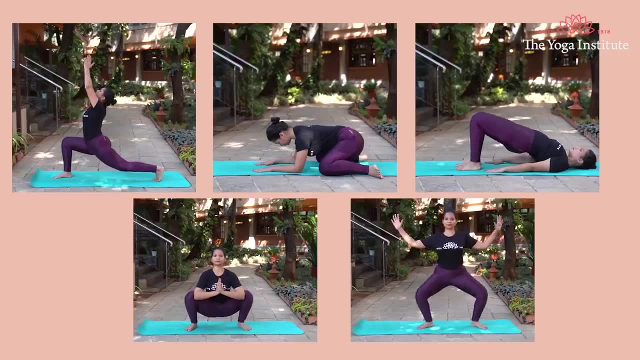 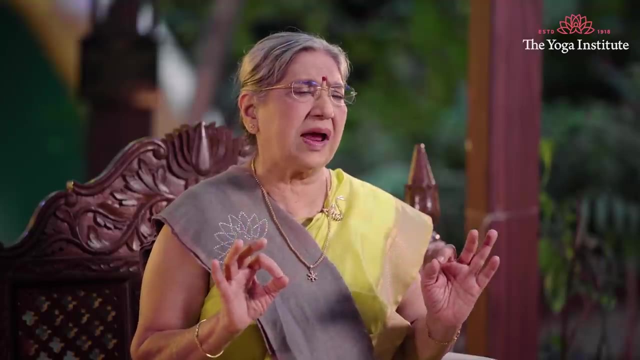 the knees. do not cross your foot. Hold the posture for 30 seconds by breathing comfortably. Release the posture. You can do this five times. Practice these five asanas to reduce the accumulated fat around the hips. Every woman should practice these five asanas regularly to increase stamina. 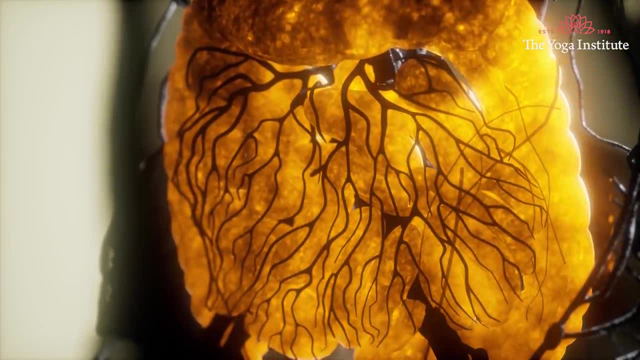 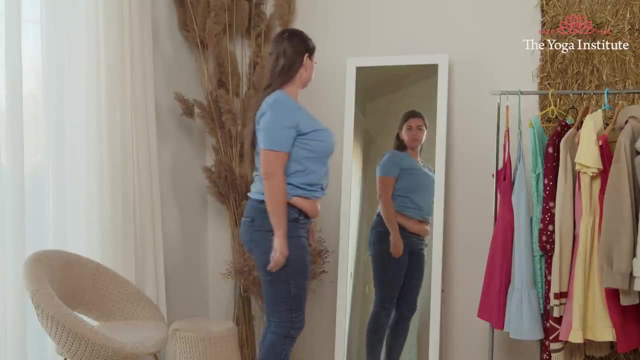 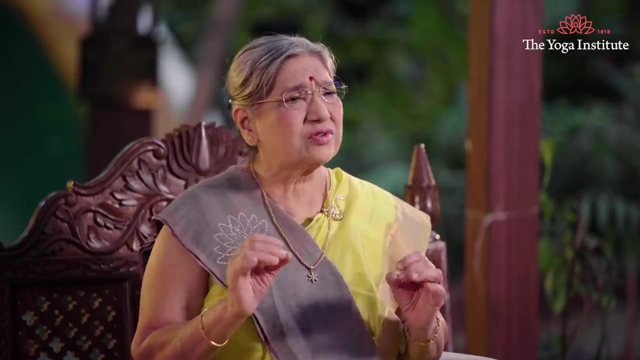 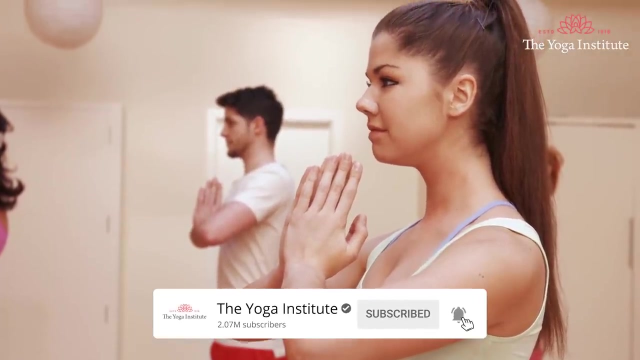 and to improve the functioning of internal organs. Understand one thing: that gaining weight is also influenced by your ideas and your emotions. Yoga is the most effective way to lose weight. It helps to improve strength and find peace of mind. Yoga promotes mind, body and emotional balance. Yoga promotes health and well being. So